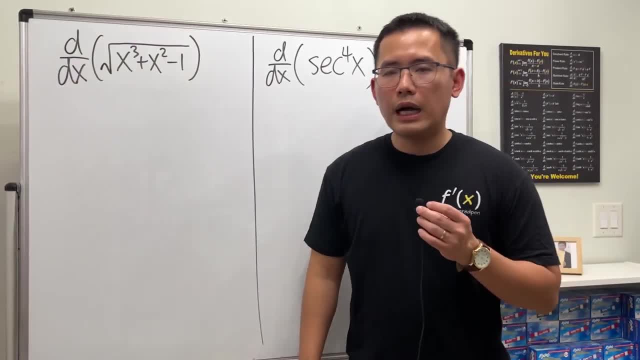 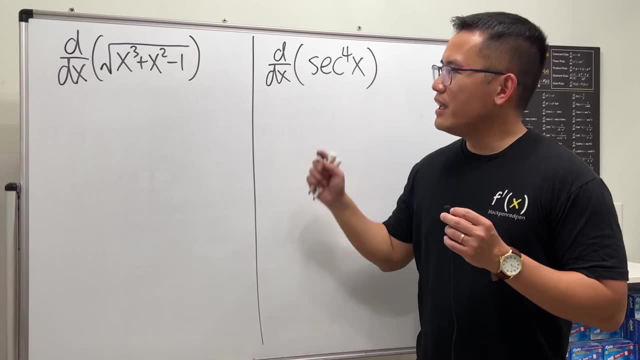 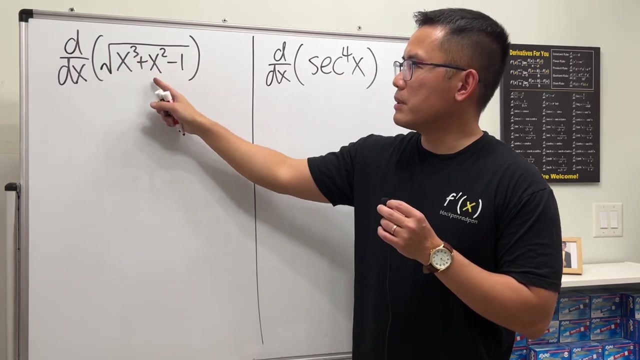 In this calculus tutorial I would like to show you guys one super easy way to understand what's going on with the chain rule when we take the derivative. And here are two examples for you guys. Let's do the first one. We will differentiate the square root of x to the third power plus x to 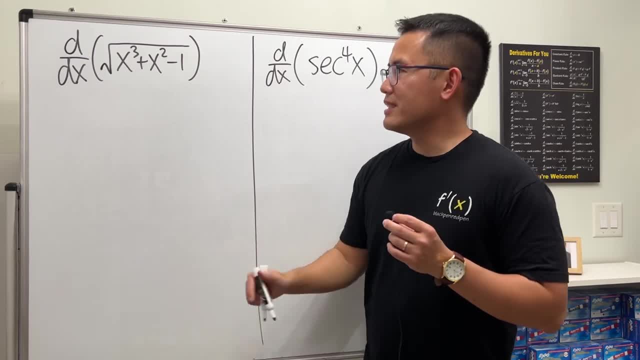 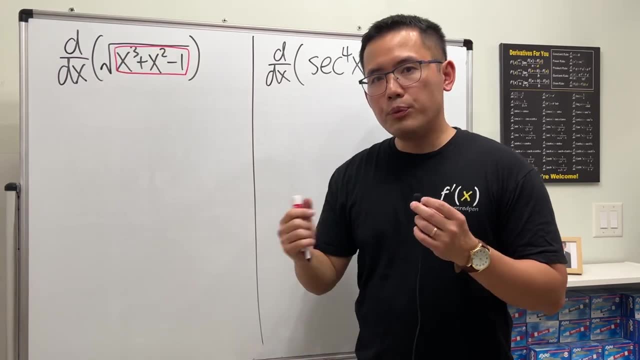 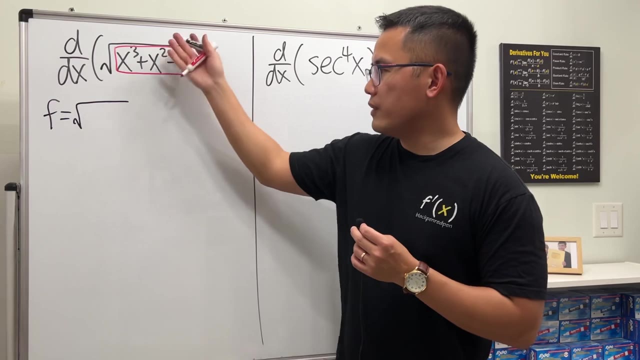 the second power and then minus one. This is how we do it. Notice that we have an inner function, which is that right Square root of this. Let me break it down for you. The outer function is a square root. I will call that f. It's just square root of a box like this, Literally a box. 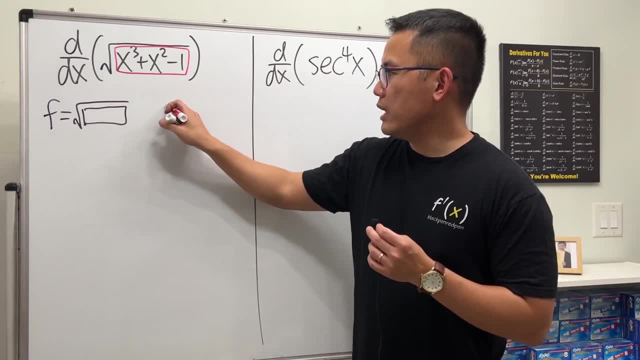 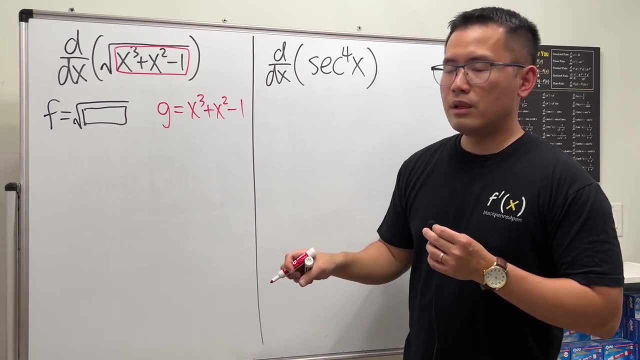 just draw a box right here And then the inner function. we label that as g and we'll just write that down, which is x to the third power, plus x to the second power and then minus one. Now we're just going to forget about this, Just focus on that. 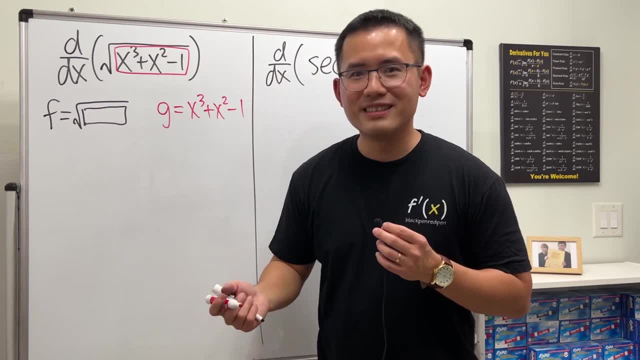 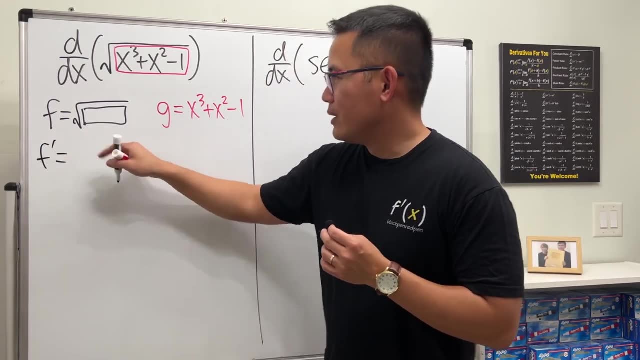 As a function, we have a square root of x to the third power plus x to the second power, and then ask yourself what's the derivative of square root of a box? One over two square root of a box. So right, here we have f prime. You can write this as to the one half power, but you will deal. 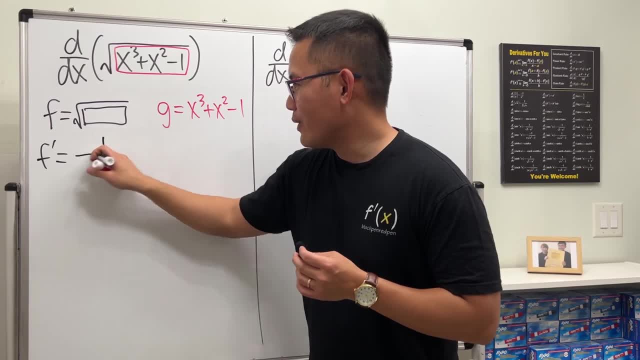 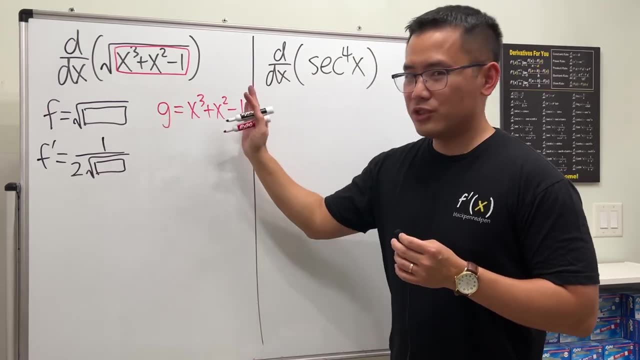 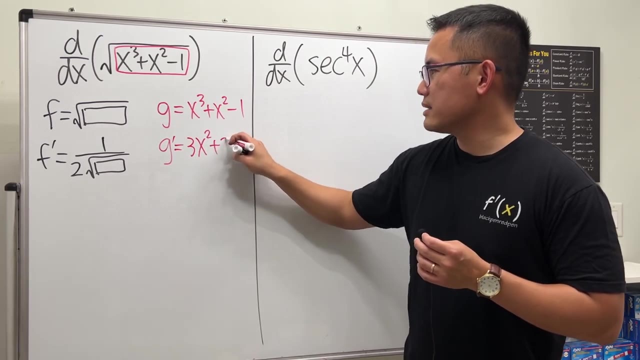 with square root a lot. So just remember it. We get one over two square root of a box right. And then let's just focus on g and take the derivative g prime. the derivative of that is just going to be three x squared plus two x. 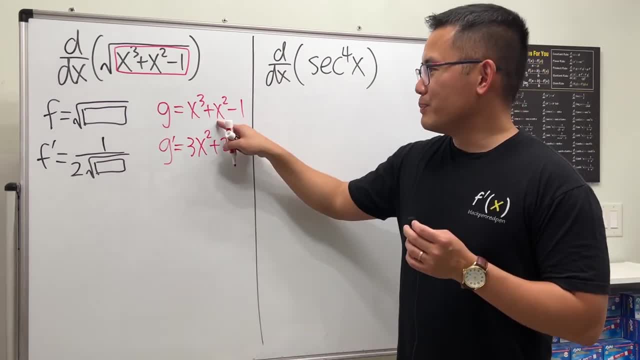 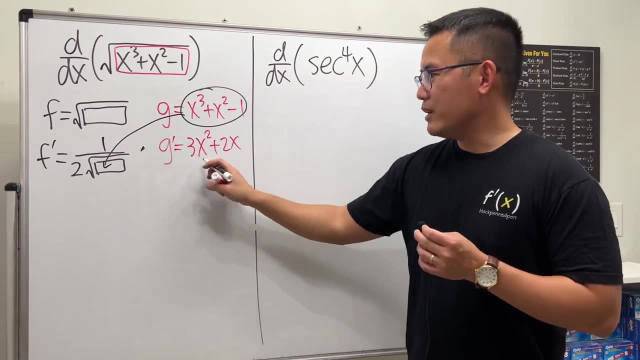 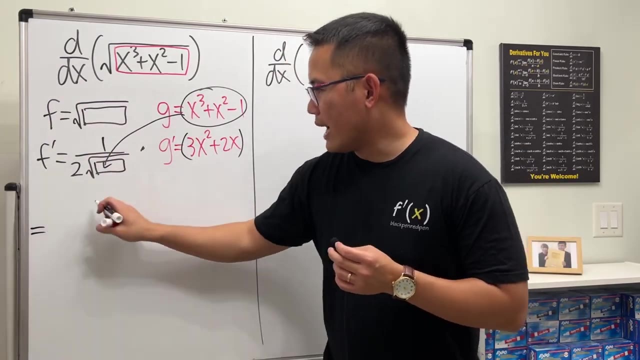 Yes, two terms. Now we are going to put g- this thing, inside of the box and then multiply by g prime. And remember it has two terms. so just put down parentheses right here. So the derivative for this is going to be one over two square root. Don't put down the box anymore, Just write that. 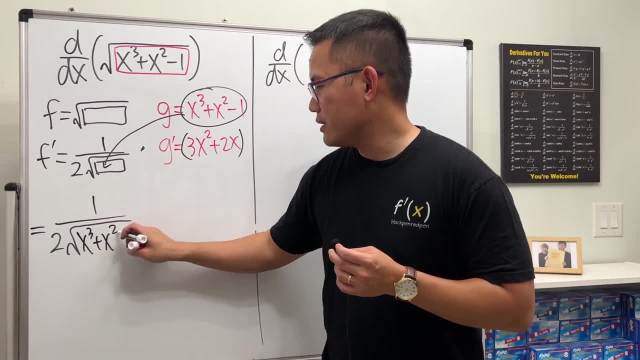 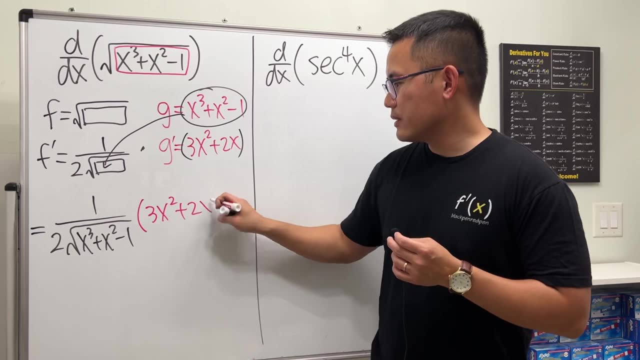 down x to the third power Plus x, squared minus one. Then that times this. So multiply by three x squared plus two x. That's pretty much it. Of course you can put that on the top and I will do that for you guys. 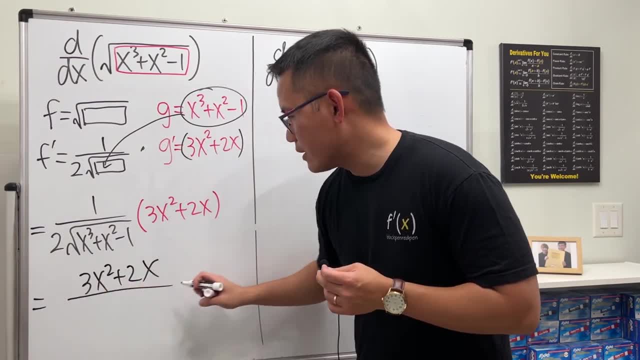 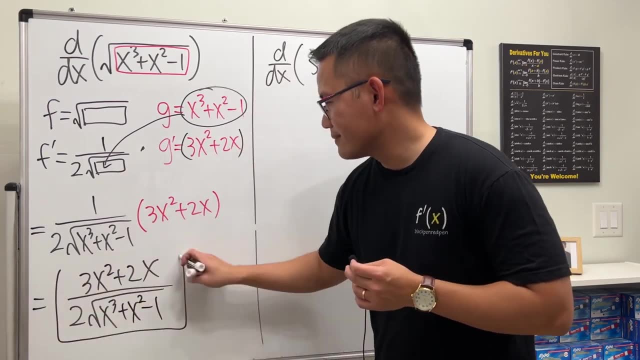 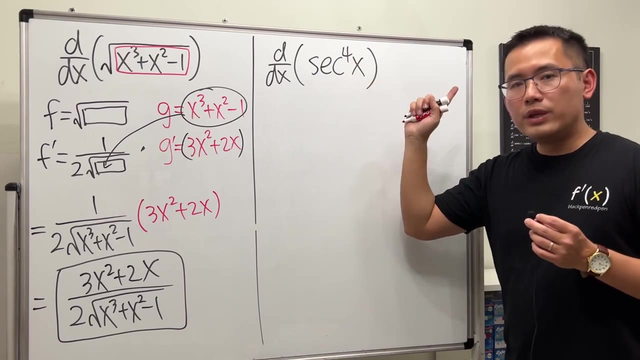 Three x squared plus two x, all over two square root of x to the third power plus x squared minus one. And then we are done. So just like that, Now for the second one, we have secant to the fourth Power, x, And we have to understand this kind of notation really well. This really means we are. 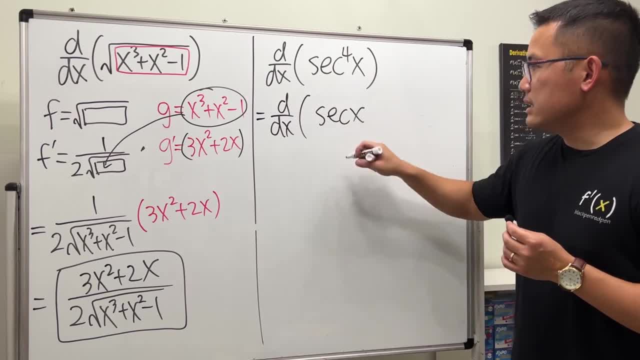 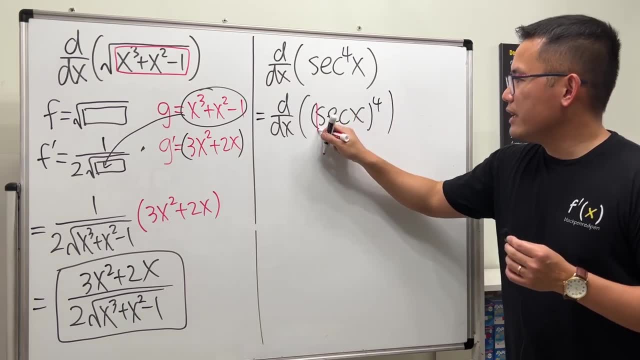 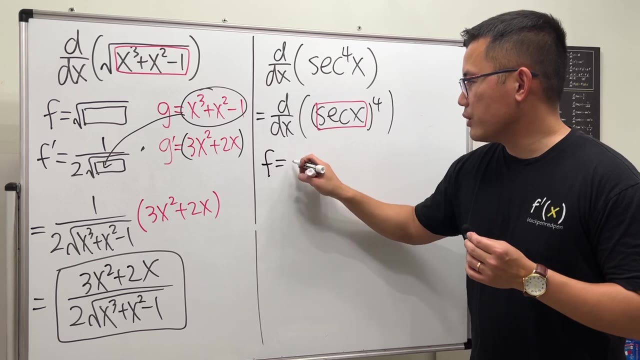 going to differentiate secant x inside and then raise to the fourth power. So we have the inlet function being secant x, So it's a box to the fourth power. So let me break it down: F is just a box to the fourth power And the inside function is secant x. 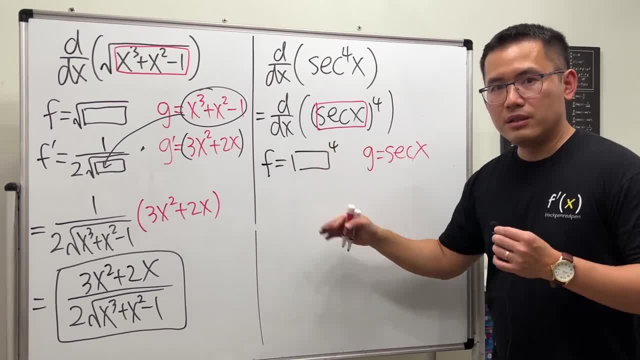 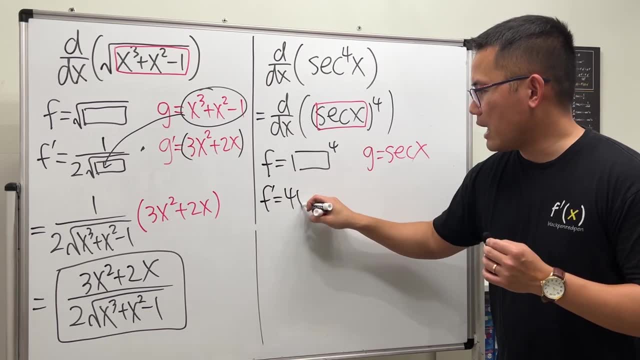 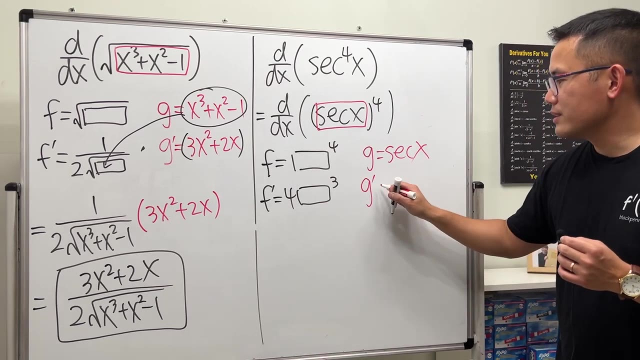 Break it down, It's easier, Less intimidating. Focus on this right here. Take the derivative: Just the power rule Four box to the third power Done. And then look here, Take the derivative: Okay, What's the derivative of secant x? Do you remember this? If you don't, here are some tips. 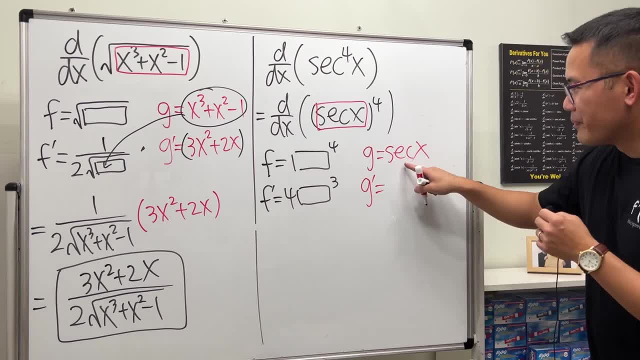 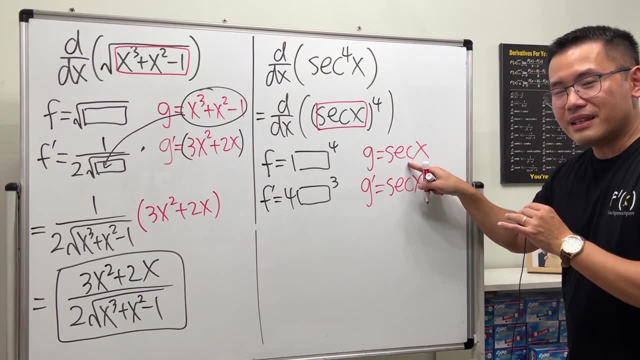 right. Check out the video. in the description I have some tips for you. The derivative of secant: it first repeats. So secant x And the derivative, And in calculus secant and tangent are best friends, So you also invite. 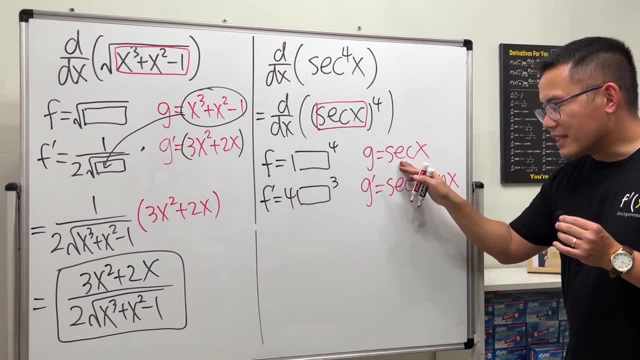 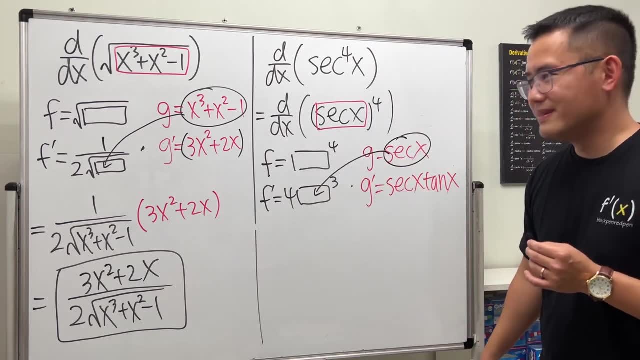 tangent right here as well. So the derivative of secant x is secant x times tangent x And then put this in the box: Multiply. You're done. So this is going to be. I'll just put an equal sign Here we have four. Don't draw a box. Draw a parenthesis for the final answer. 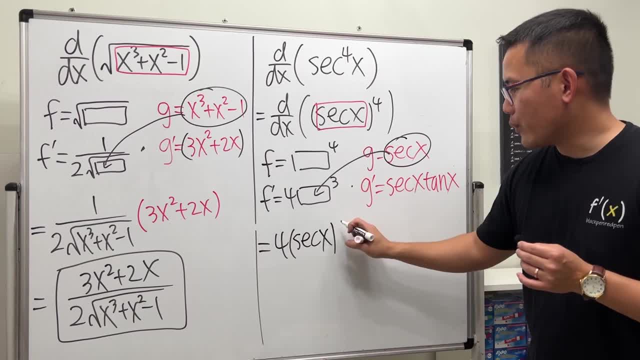 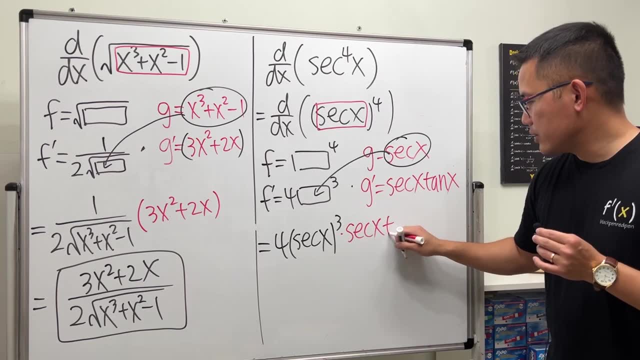 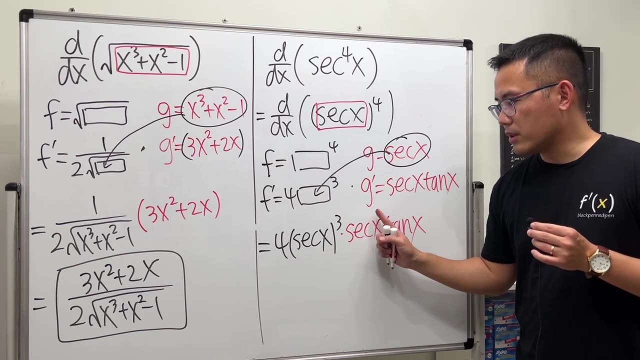 Write down secant x to the third power. That's the first part. And then we multiply by this Secant x and then tangent x. Finally, we see that we have secant x to the third power and then secant to the first power. 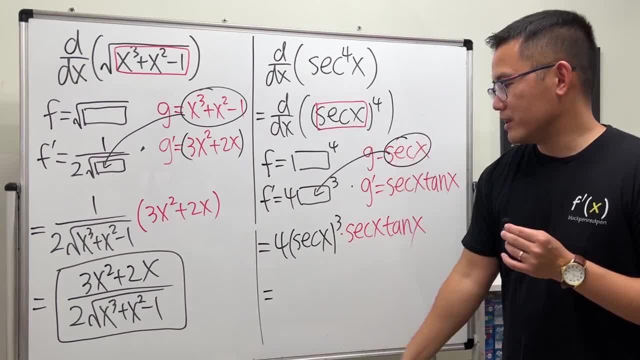 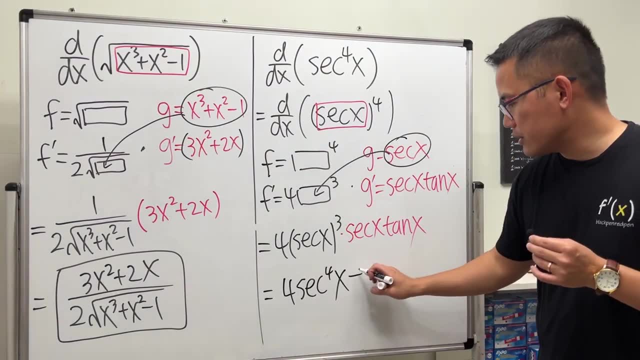 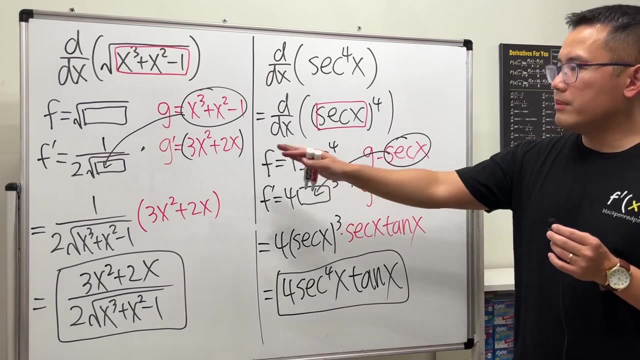 These two together, we can write this to the fourth power, So we have four, and then secant to the fourth power, x, And then we attach that tangent x And we're done. So hopefully this right here can make the chain rule more clear, And of course I know chain rule.